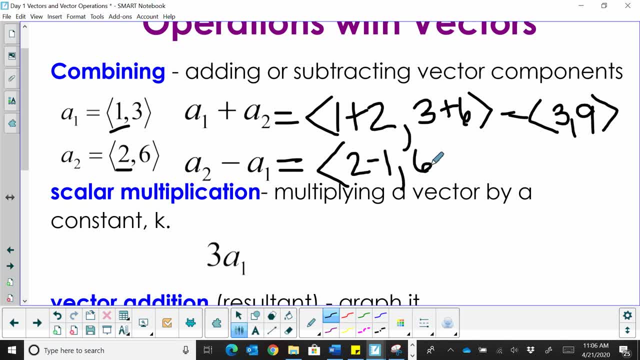 vertical component And then the vertical component. we're going to take 6 minus 3.. And our resultant vector would then be 1 comma. what's that? 3.? So the resultant vector is 1, 3. Very, 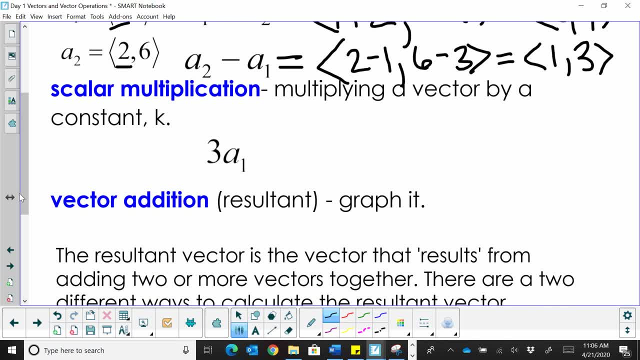 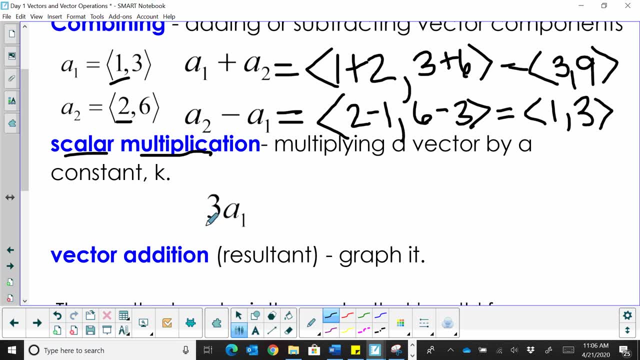 very simple to combine with adding and subtracting. Now let's talk about scalar multiplication. There are a couple different ways to multiply with vectors, But the first one is just scalar. So you're going to multiply The vector a sub 1, the first vector by 3.. So we're just going to take 3 times the vector 1,, 3,. 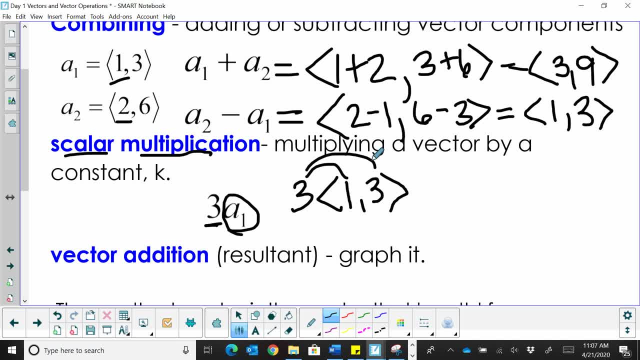 which is a scalar. So we're just going to distribute and basically dilate that vector from the position 1, 3, 2, 3, 9.. And that's how you apply that scalar multiplication: You just multiply by the constant. So we're going to take 3 times the vector 1, 3, which is a scalar. So we're 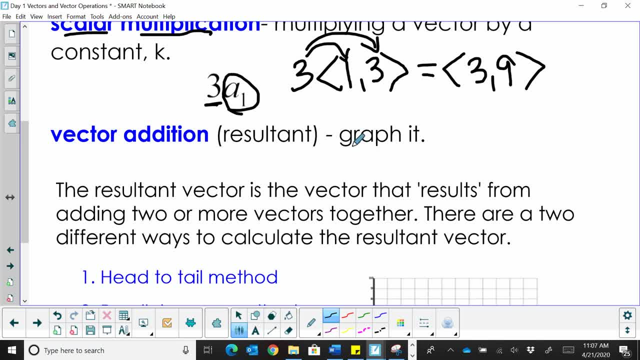 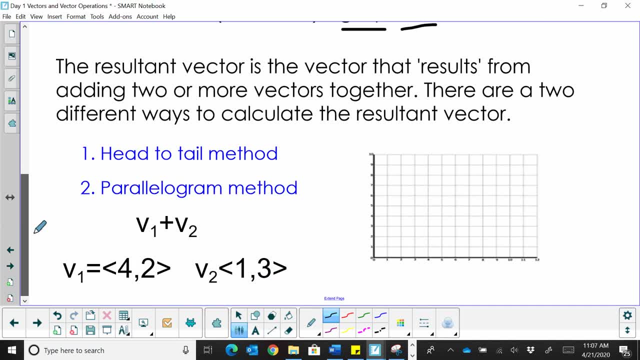 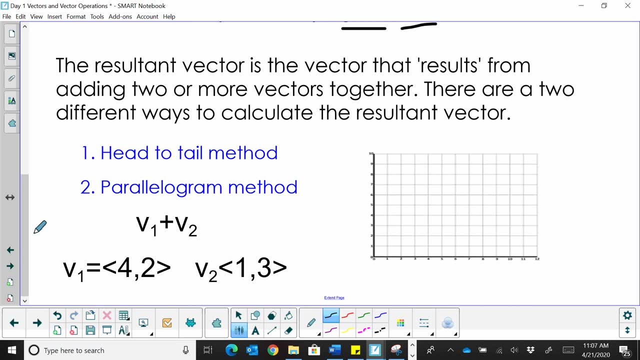 just multiplying by the constant K. Now let's look at vector addition from more of a graphing approach And we can see the same resulting vector with graphing. So the resultant vector is the vector that results from adding two or more vectors together, And there are two different ways. 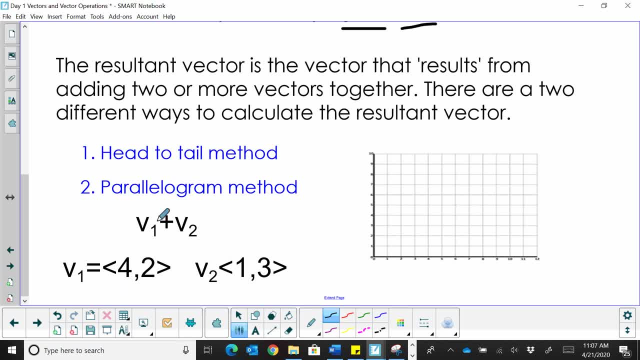 to calculate that resultant vector. So let's say we're going to take vector 1 and vector 2, v1,, v2.. And we're going to add those together. So what I'm to do graphically is I'm going to start using the head to tail method, So I'm going to draw first. 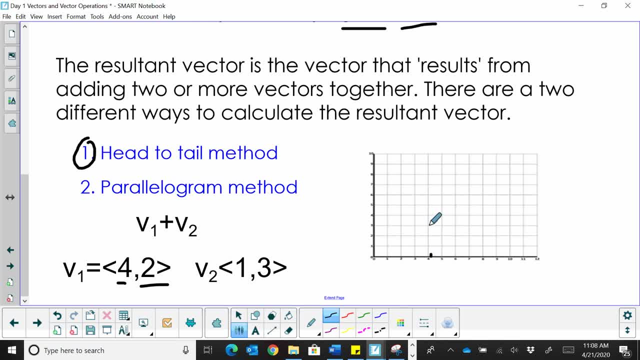 the vector 4, 2.. So that means I'm going over 4 and up 2.. So my first vector from standard position would be this vector: There's 4, 2.. I'm going to then add to it the vector 2, which is the vector. 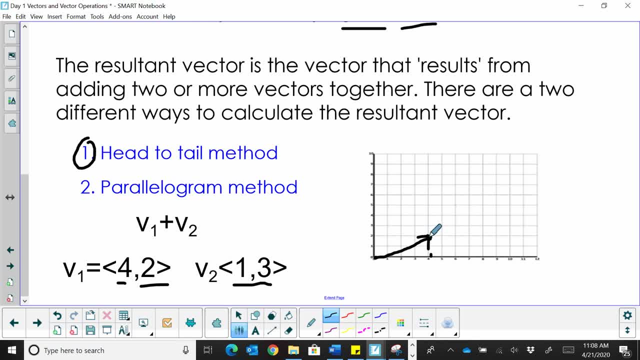 1, 3.. So at the tail end of the first vector, I'm now going to draw my second vector. So I'm going to go over from the end of this one, I'm going to go over 1 and up 3 and draw my second. Oops. 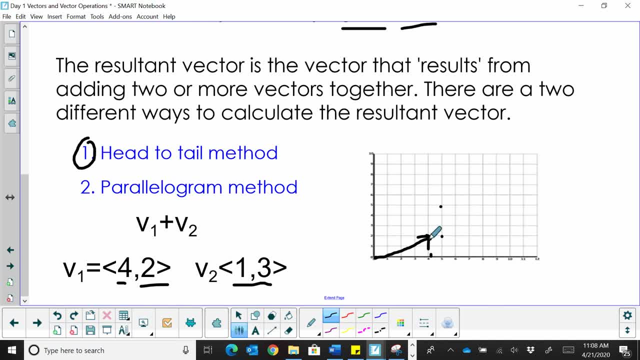 that didn't draw very well. Let's undo that one and draw this a little straighter. Well, that wasn't much straighter, but there's my ending result. So there are my two vectors added together. So what is the result? 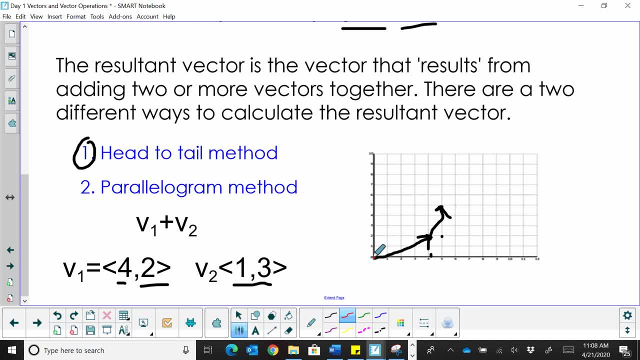 Of that vector. I'm going to draw this one in red, from the beginning where I started, to the very end where I ended adding those two together. That is my resulting vector. So the red vector is my resulting. So what if I just created what is the component form of the red vector? 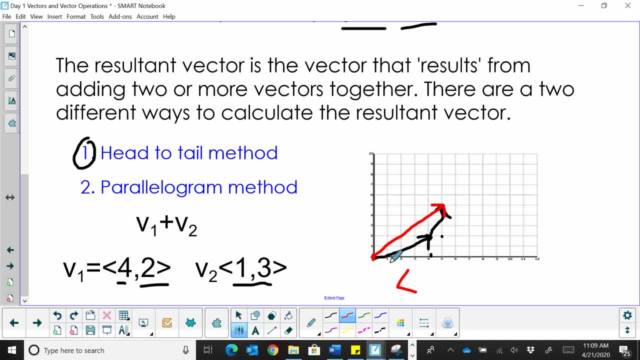 Well, the component form is 5,. right, I've gone over 5 in my horizontal direction And I've gone up 5.. So my resultant vector is the vector 5, 5.. And that is the head-to-tail. 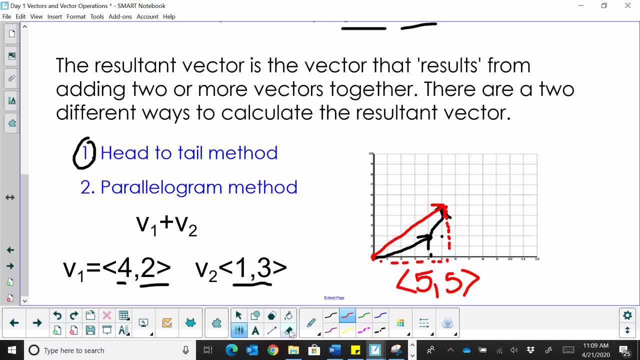 method on adding two vectors together. Now let's look at the parallelogram method. This is very helpful, especially when you get to the bigger vectors. How can you calculate this with a parallelogram? Well, what you're going to do is you're going to start. this time I'm going to use some actual 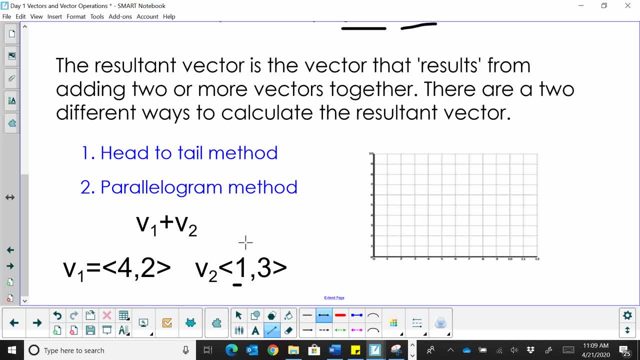 errors. You're going to start and draw both of the vector 1 and vector 2 from the origin. So I'm going to start 0, and I'm going to draw the first one from the origin and there's 4, 2.. Then I'm 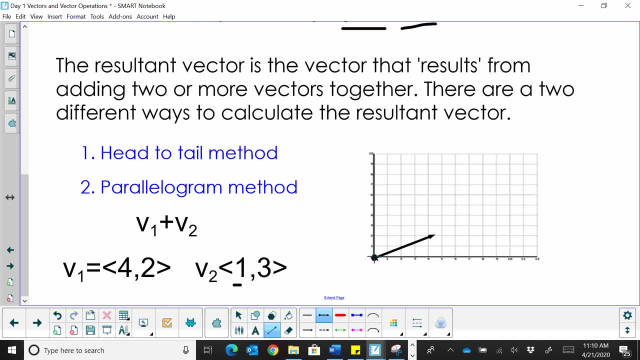 going to draw the second vector- 1,, 3, also from the origin. Okay, Now, what I'm going to do is I'm going to create a parallelogram, So I'm going to go over here and basically just copy this: 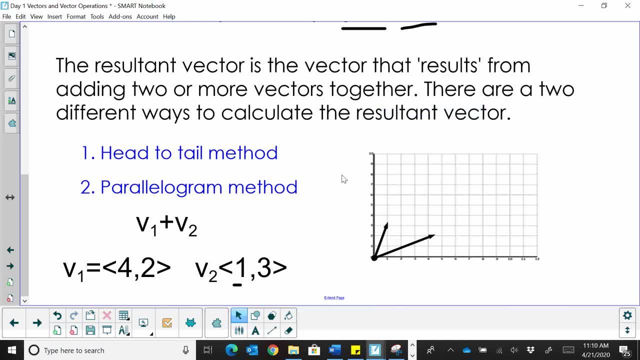 vector. So I'm going to copy it and I'm going to paste it And I'm going to draw this vector. Let's grab it here And draw it here. And then I'm going to also copy this one And I'm going to also copy this one.